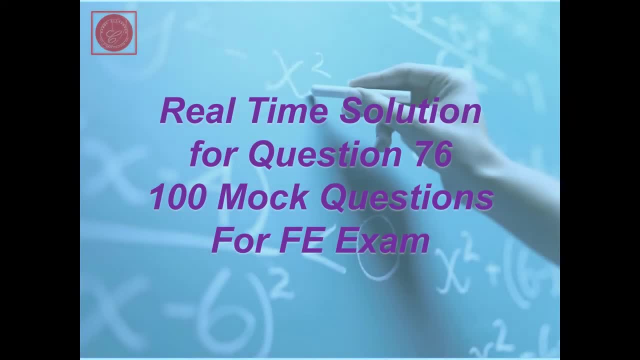 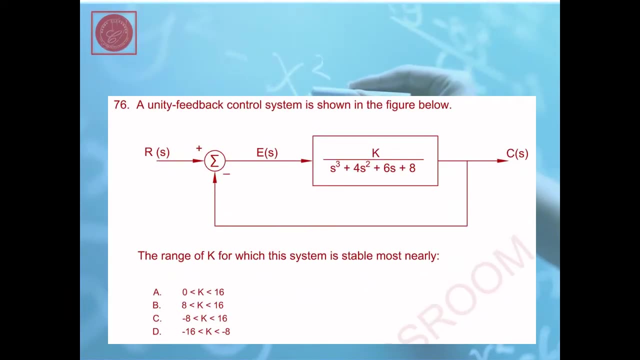 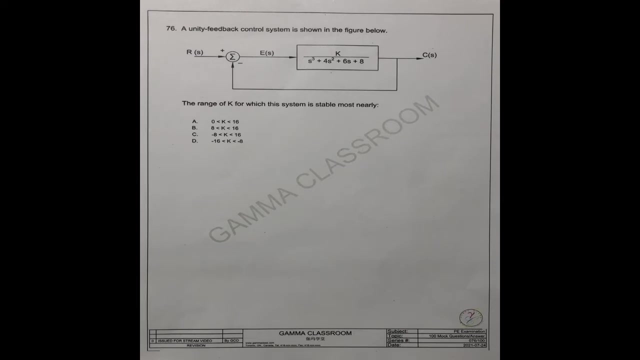 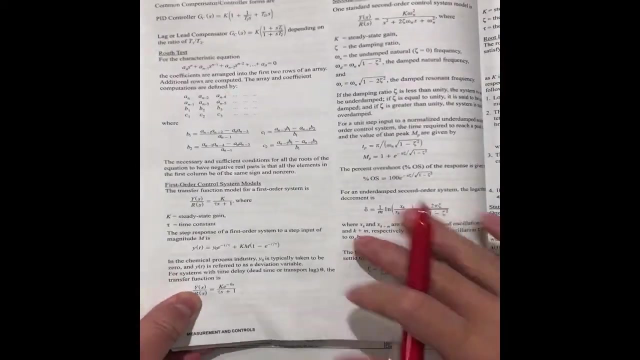 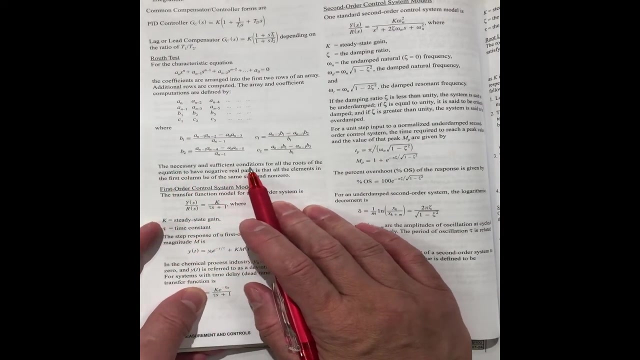 A unity feedback control system is shown in the figure. below the range of k for which this system is stable most nearly. what number? ABCD? When this question is talked about the control system stable, we can find the information in the page 112.. They have the loss test Here, the necessary and sufficient conditions. 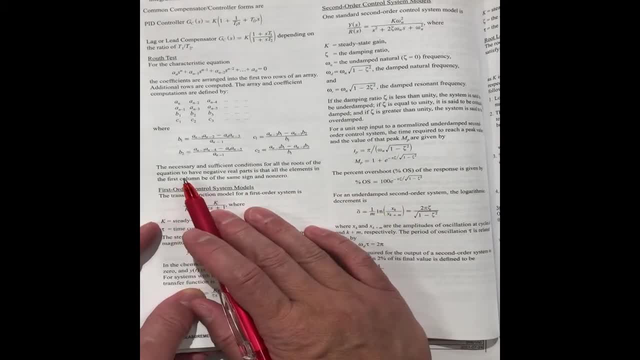 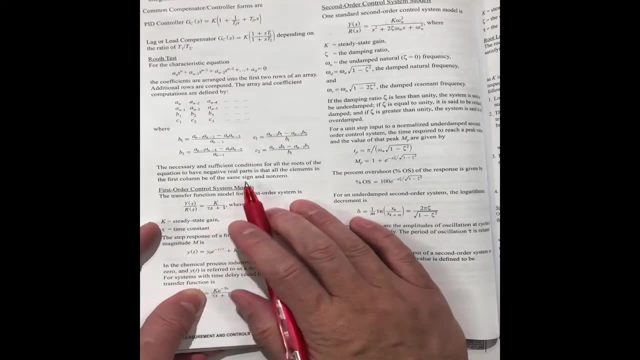 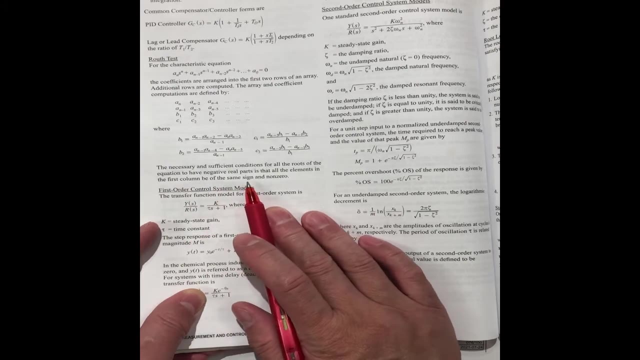 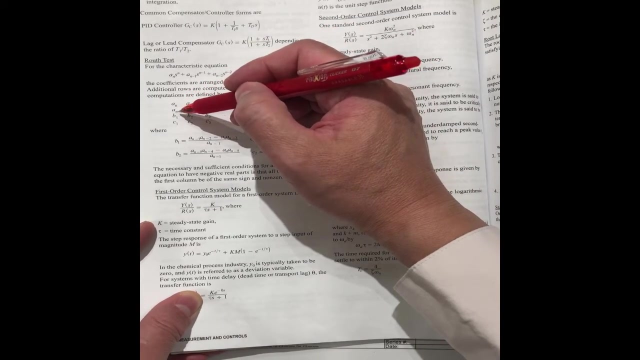 for all. the routers of the equation are as follows: The equation to have negative real paths. Negative real paths means stable. The existence is stable Is that all the elements in the first column be of the same signs and non-zero. This means in here AM, AM minus 1, B1, C1,. all these current elements should be the same. 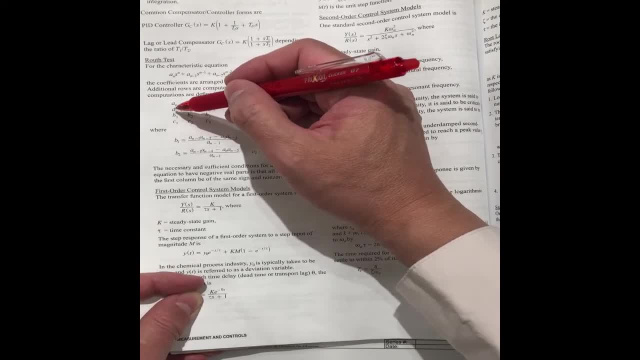 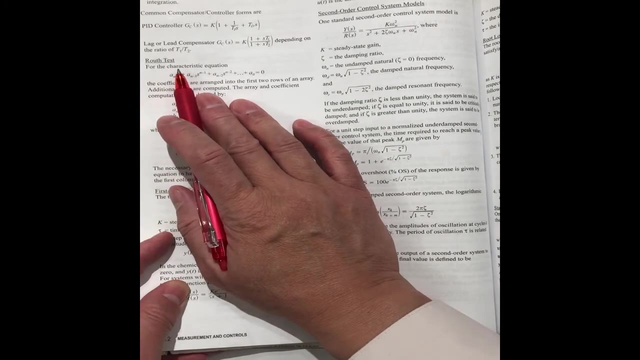 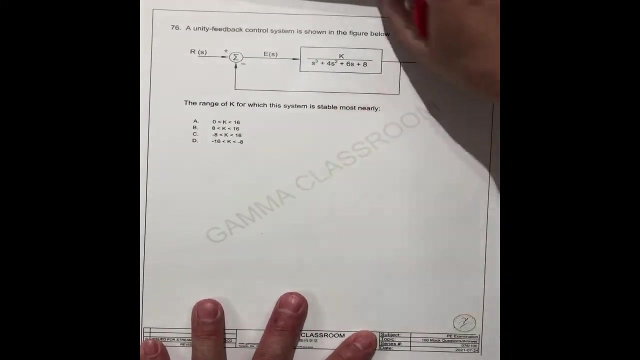 signs Positive or negative? No signs changes. If it's positive, all the positive. If it's negative, all are negatives. So we know the condition. So for now, we need to find what the characteristic of this control system is For this one. so we have the formula. 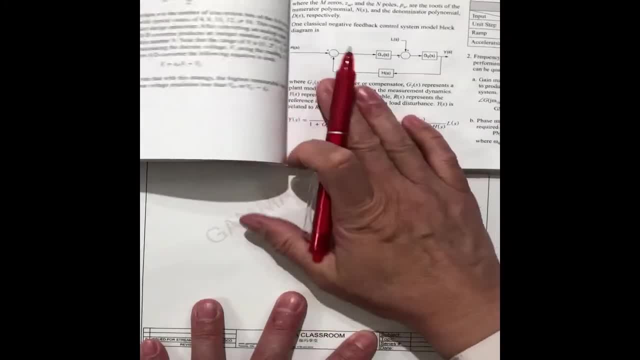 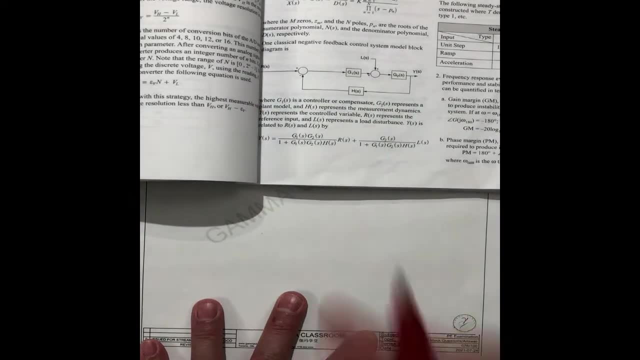 We have the definition here: This, This, This, This, This And this one And this one here. This code is called the digital gettin in the 줘-mé-particle system. This is the classical negative-feedback control system or EALQ-fy BI control system, but also. 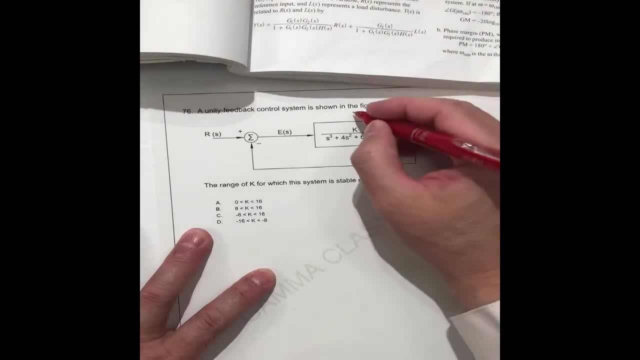 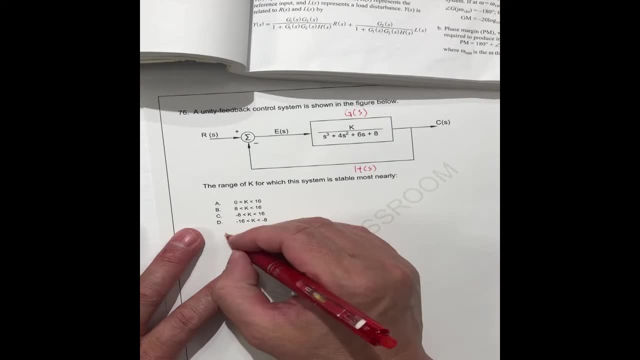 model. So we just follow this model And we use this code GS. here we call the HS. So cs divided byavier is equal to this: G1.. G1.. G2.. G3., G4., G24.. 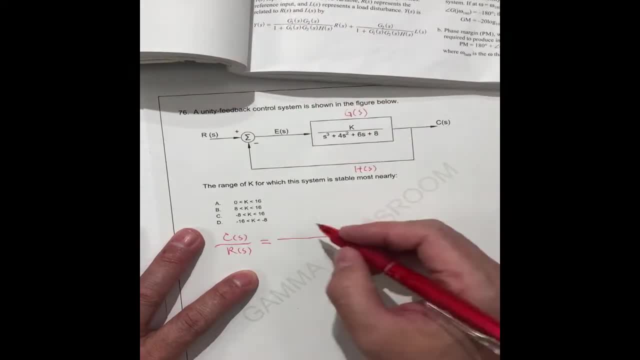 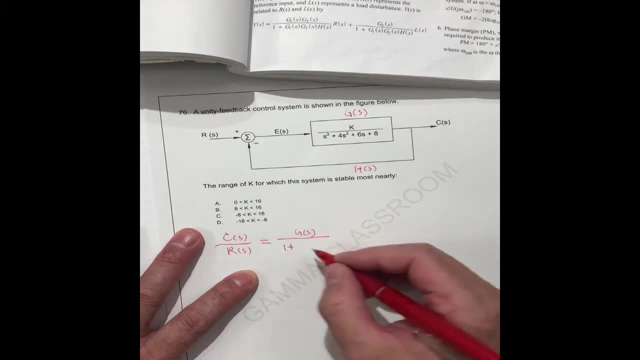 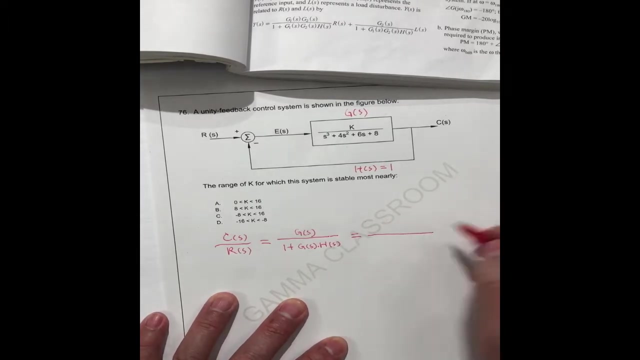 G5. And we see that today we can demand numbers Broadly speaking, this normal memory that we will fall in. this equation入 a is equal to, based on some very simple rules, just gs, gs and 1 plus gs times hs. We know hs is the unit equal to 1.. So we can put the 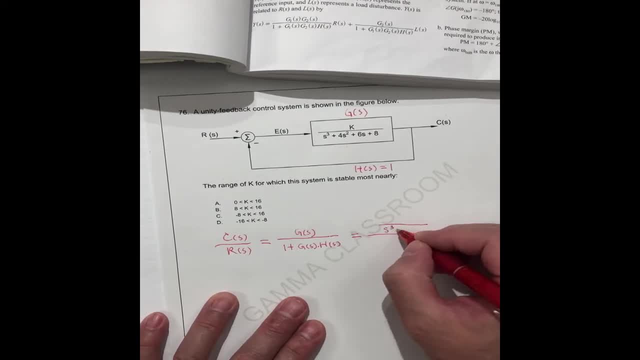 formula here inside: This is hs plus 4s squared plus 6s plus 8.. This is k. And here is 1 plus gs, This one. So hs plus 4s squared plus 6s plus 8.. This is k. 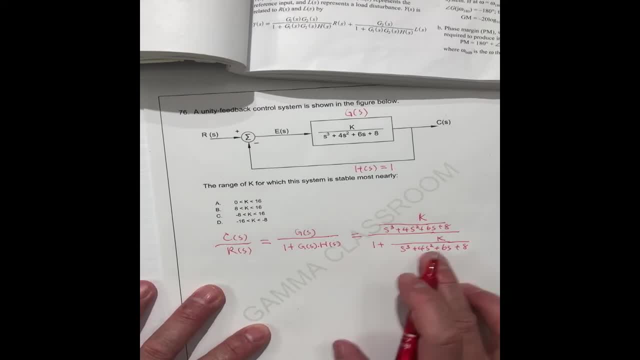 We just simplify: times this one And we can cancel this. Get this one. See, this is hs is equal to 4s squared plus 6s plus 8.. This is hs squared plus 4s, 6s plus 8.. This is: 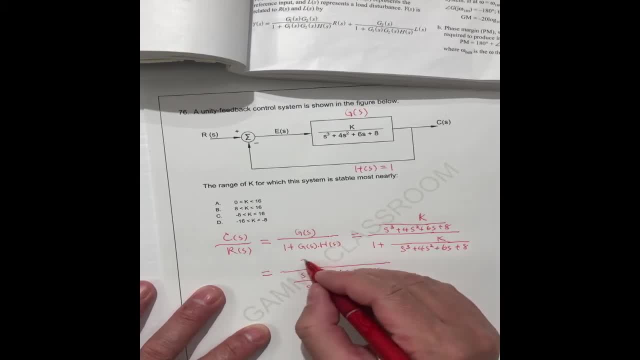 k. This is the same. hs is equal to 4s squared plus 6s plus 8.. This is k. We know this is the same. We can cancel each other, So we can get the number is hs plus 4s squared plus. 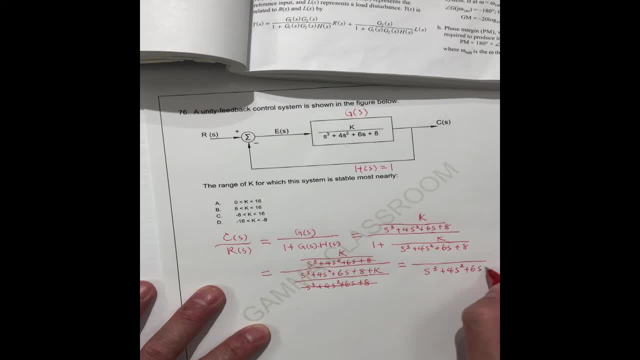 4s plus 8.. hs squared plus 6s plus 8 plus k And k, So this is the characteristic equation. So this is hs 3 plus 4s, squared plus 6s plus 8 plus k, equal to 0.. So we can use the loss. 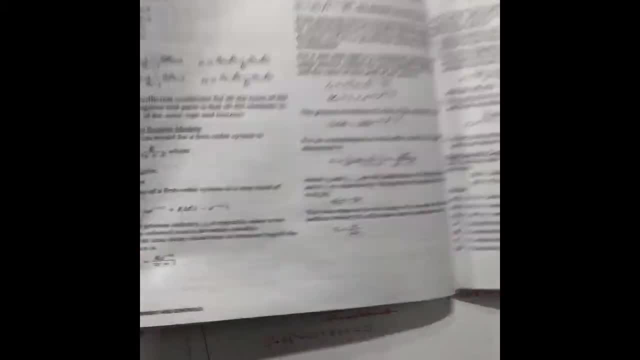 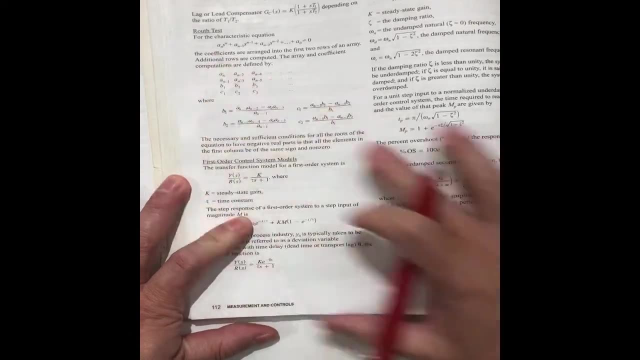 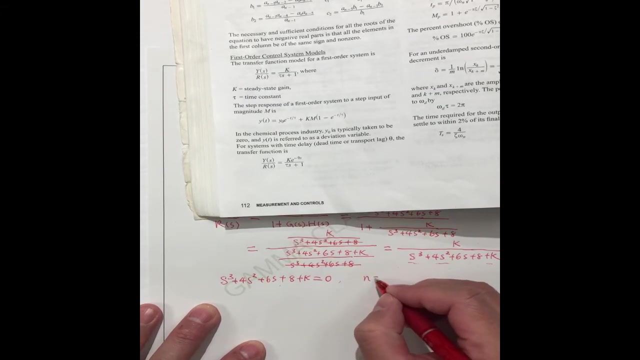 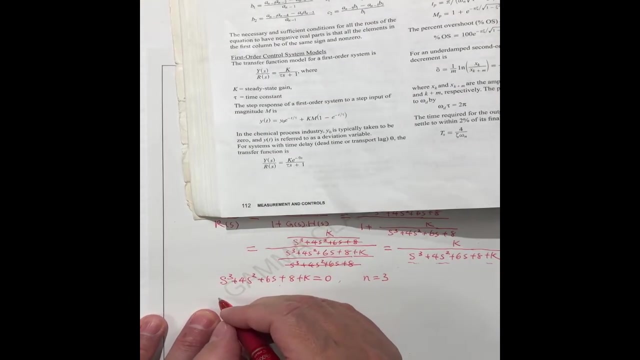 test formula. Formula here: This one A. You see this: in this equation, The highest order M is equal to 3.. Right M is equal to 3.. So A A, 3.. Use this one A 3.. 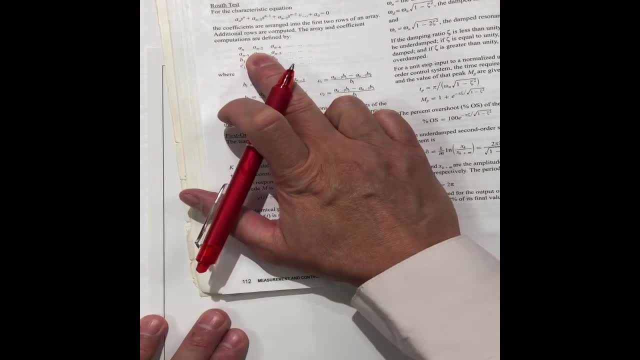 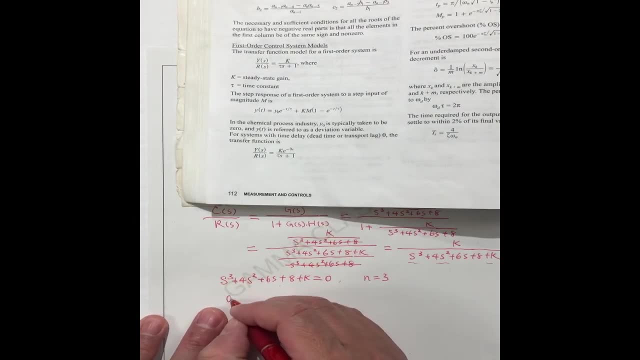 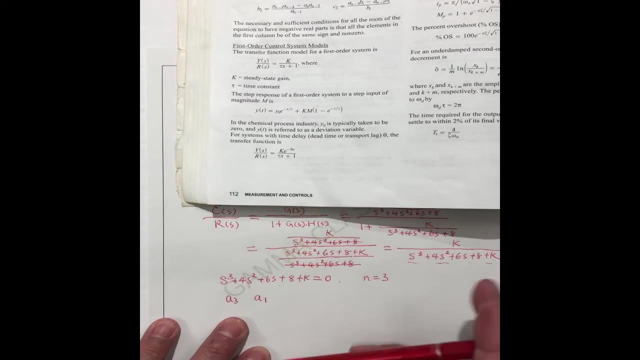 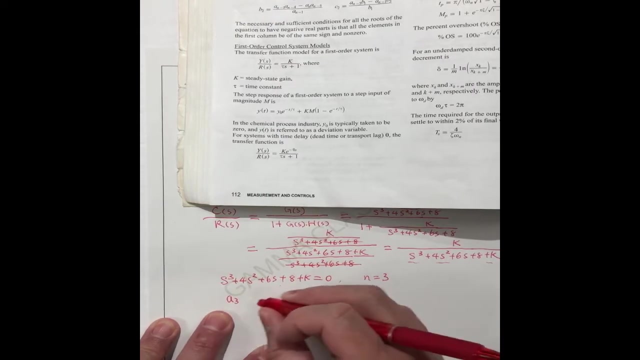 M minus 2 is A 1.. So this is the first one: M A 3. A 1 is equal to what number A 3 should be equal to? Oh, A 3 should be equal to 1.. Right. 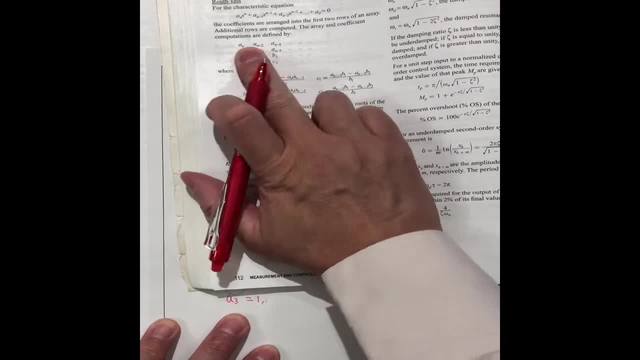 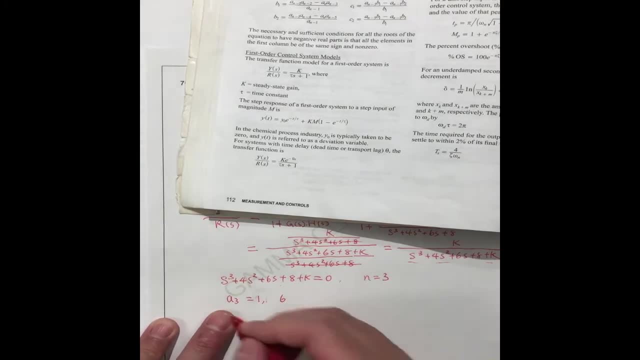 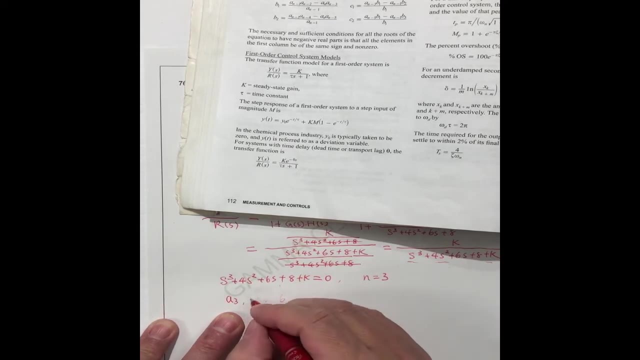 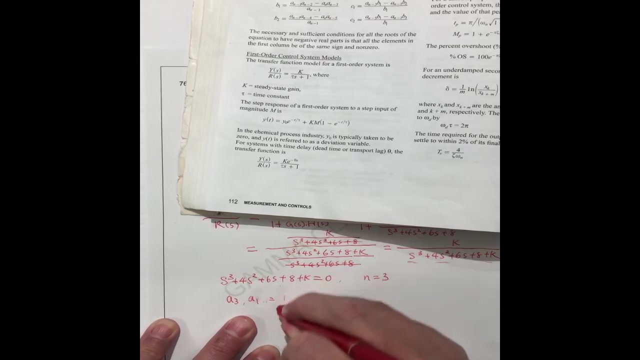 The first rules. This one, 1 and 1 is 6.. Should be A 3, A 1.. Like this, A 1 is equal to 1.. This is 1.. A 3 is this one, A 1 is 6.. 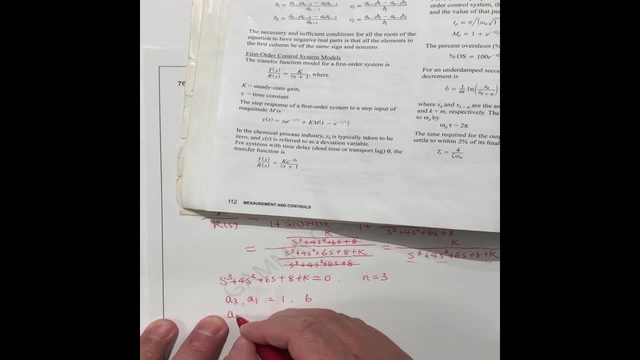 This is A 2, A 0.. Which one, A 2, is 4.. A 2 is 4 here. 3 2 1, 0.. Right, A 0 is this one: 8 plus 8 plus k. 8 plus k. How about the B 1?? This is B 1 here. This is B 1 here. 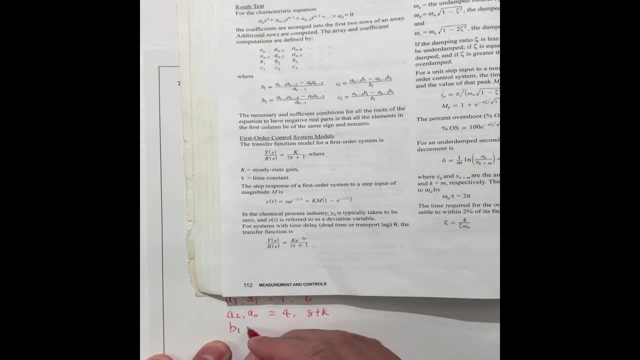 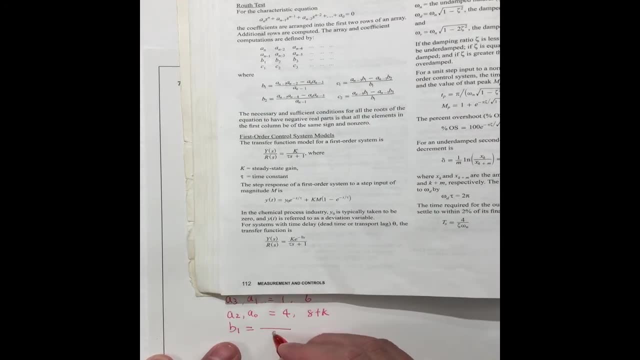 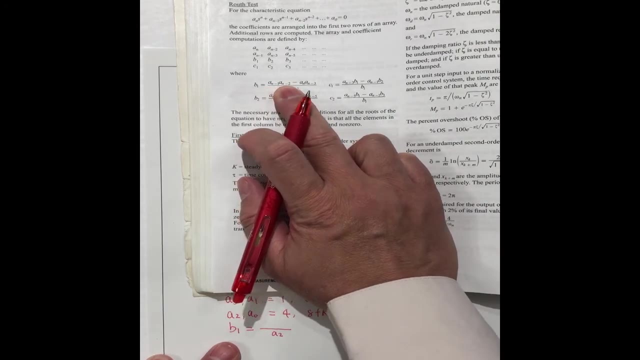 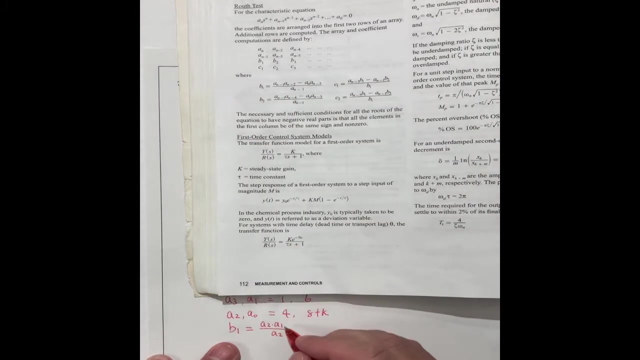 This is B: 1. Equal what number A? 3 minus 1 is A, 2. This is A. 2. This is A. 3 minus 1 is 2.. 3 minus 1 is A: 1. So A, 2. A, 1. This is A. 3 minus A. 3. This is M minus. 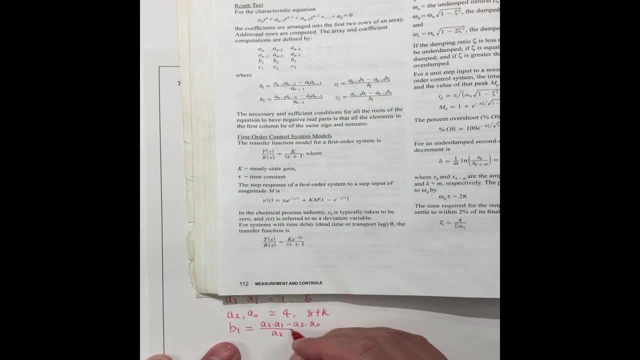 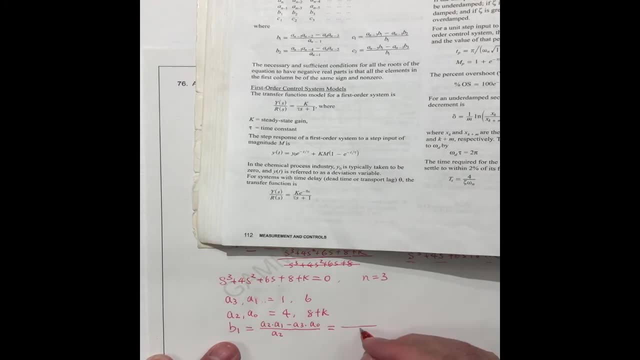 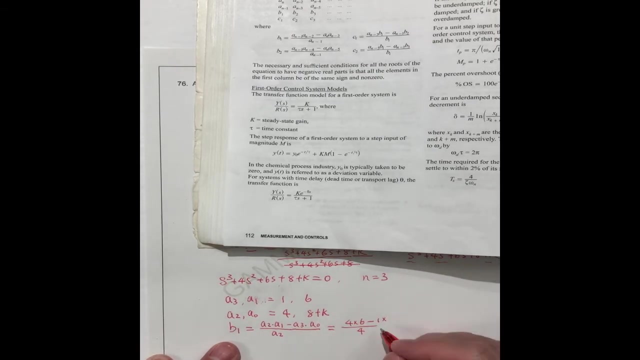 3.. This is A 0.. Should be equal to A 2. is which one A 2 is 4.. A 2 times A 1. A 2- A 1 is 4 times 6.. Minus A 3.. A 3 is 1. Times A 0.. 8 plus k: This is M, minus This is A. 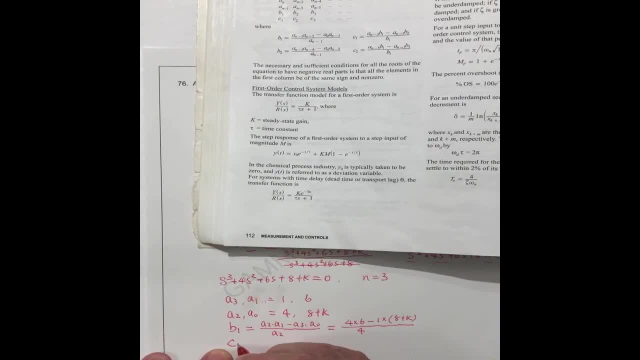 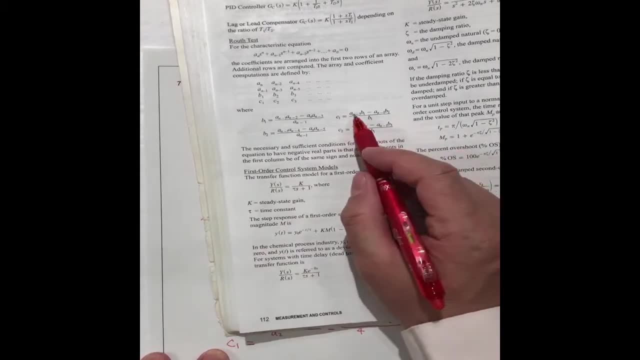 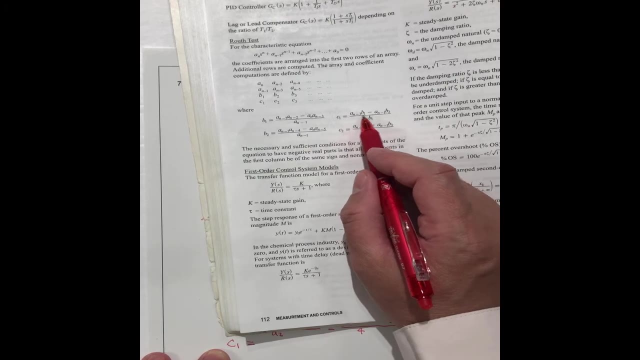 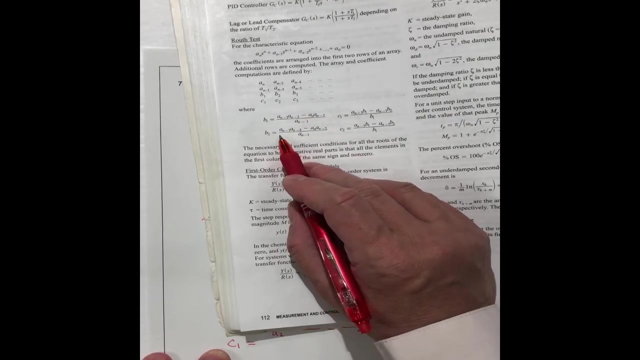 1. How about C 1?? C 1. Here C 1, because this is A M minus 3.. A M minus 3. A 3 minus 3 is A 0. This is B 2. B 2 is equal to 0.. We have no B 2. Because B 2 is A 3. No M 3. 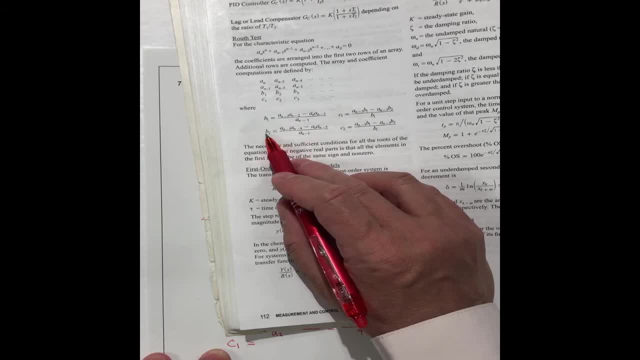 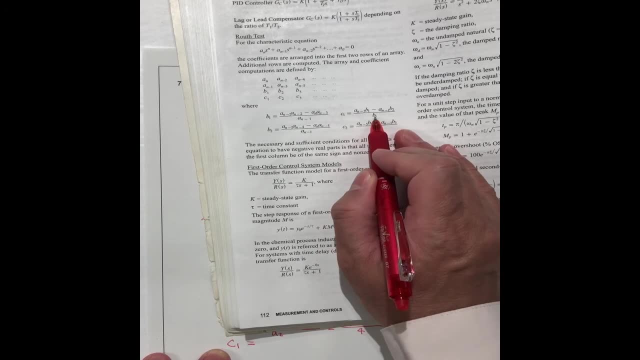 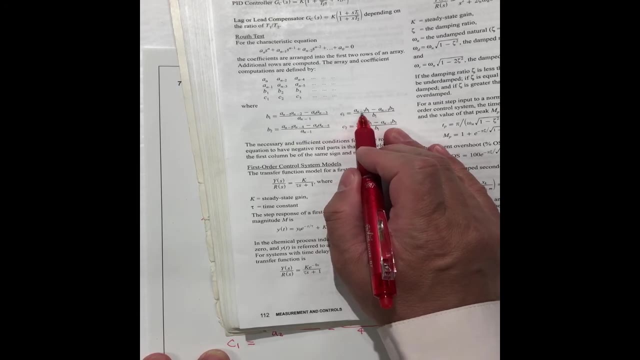 because the maximum is 0.. Number 3. So there is no B 2. So B 2 is 0.. So B 1. A M, This is B 1.. B 1 minus Divided by D 1. We cancel the B 1.. So C 1 is equal to A M minus 3. Equal to A 0. C. 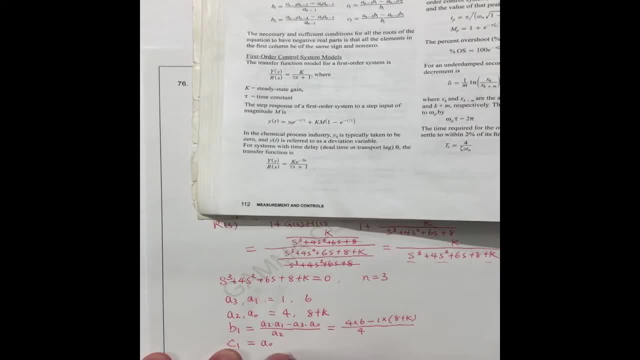 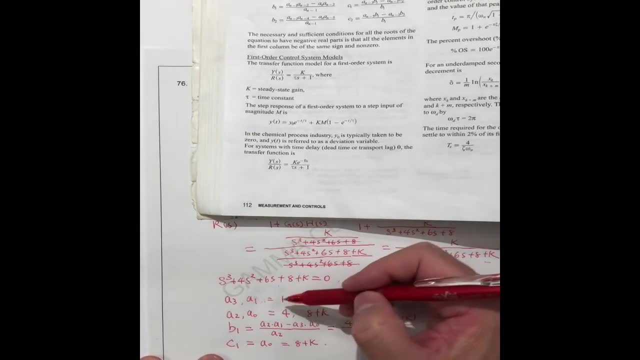 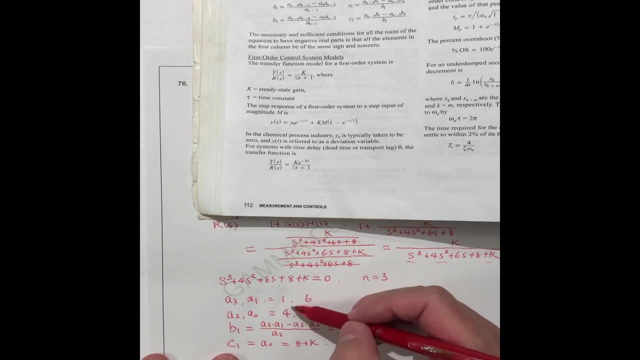 1 is equal to A 0.. What is A 0? A 0 is 8 plus k. So you see in this curve 1,, 2,, 3,, 4.. All This is 1.. This is 4. The positive Positive. So this one should. 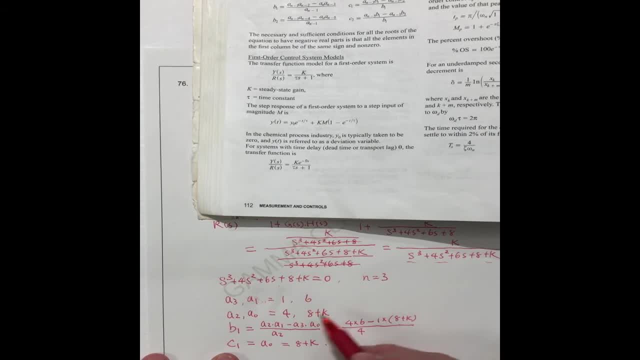 be positive. This one should be positive If all condition is satisfied, So this system will be stable. So this one should be greater than 0.. This one should be greater than 0.. So, from here, Move this 4 out 24.. Move this 4 out 24.. Move this 4 out 24.. Move this 4. 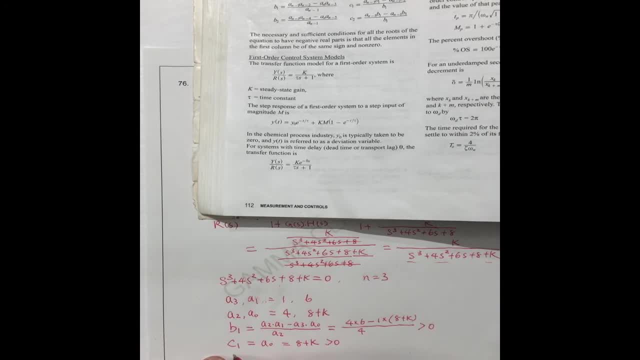 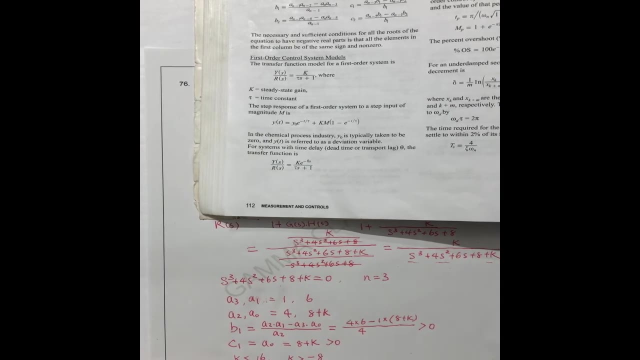 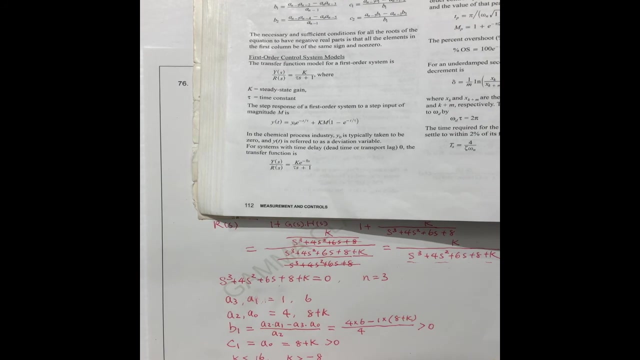 out This: 8.. So k is less than 24 minus 8 is 16.. So from this one From here, k is greater than minus 8.. So the range for the k should be k less than 16. greater than minus. 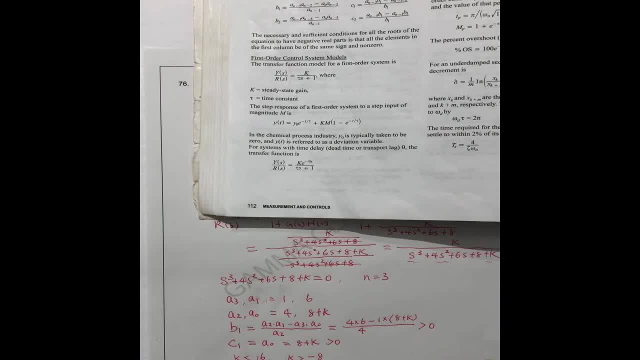 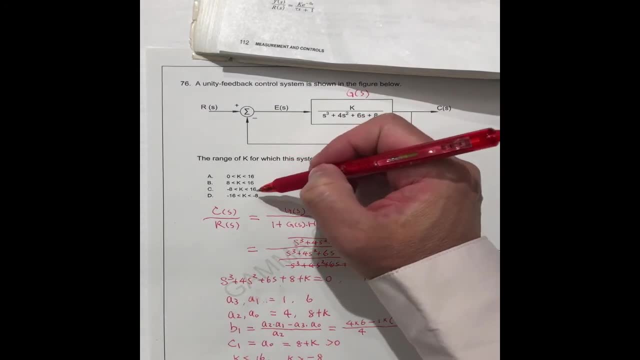 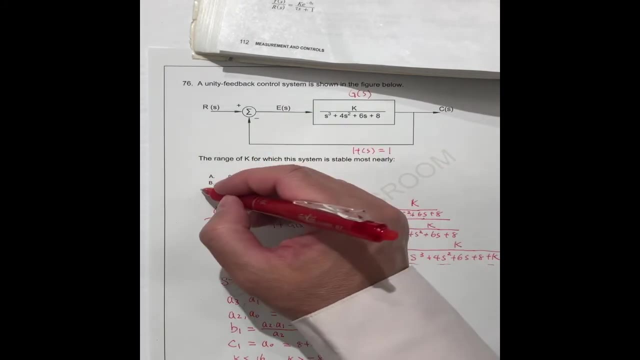 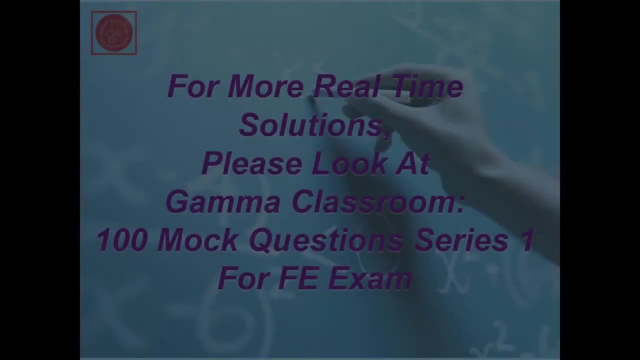 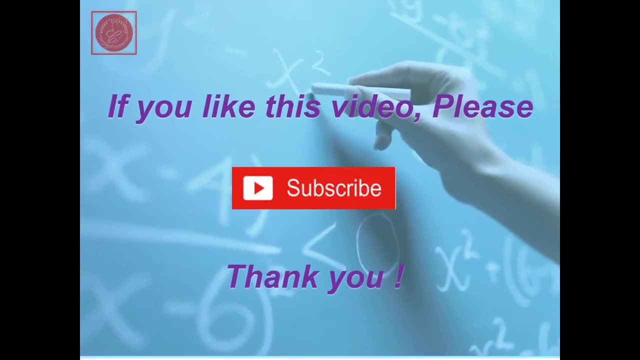 8.. So we can check the answer. The answer should be C Right Minus 8.. Less than 16.. C Should be C. Correct answer: C- Correct answer. C- Correct answer.